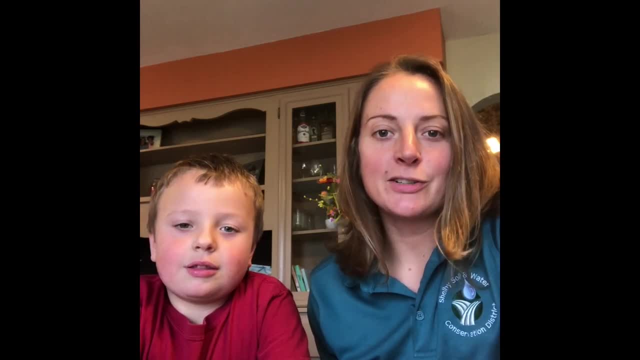 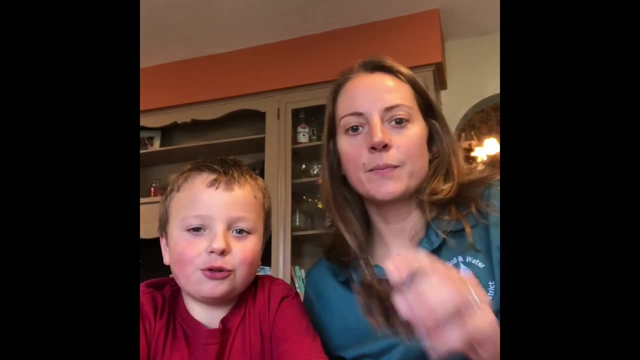 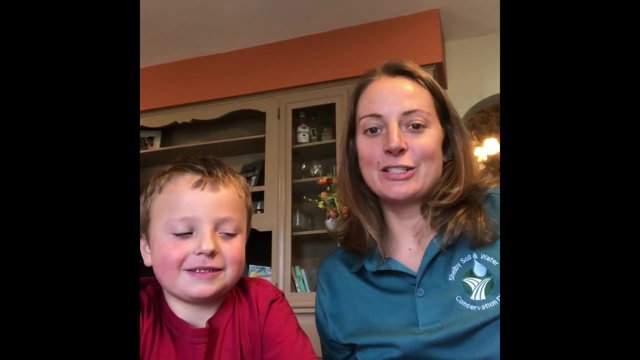 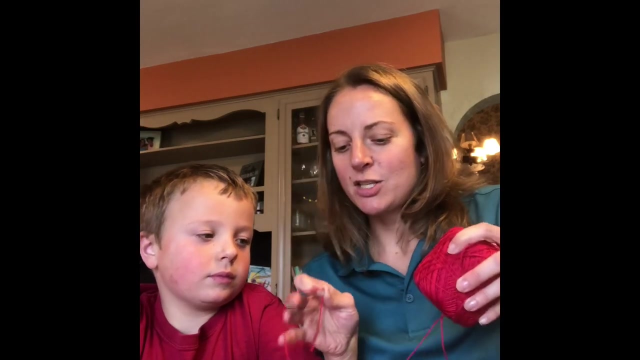 you have at home pretty easily, okay, So the first thing you're going to need to find is either a toilet paper roll or a pine cone. The next thing you need to do is cut some string or yarn to put through the pine cone or toilet paper holder. okay, So I'm going. 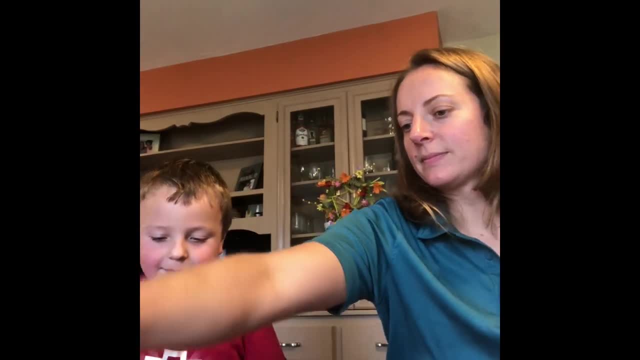 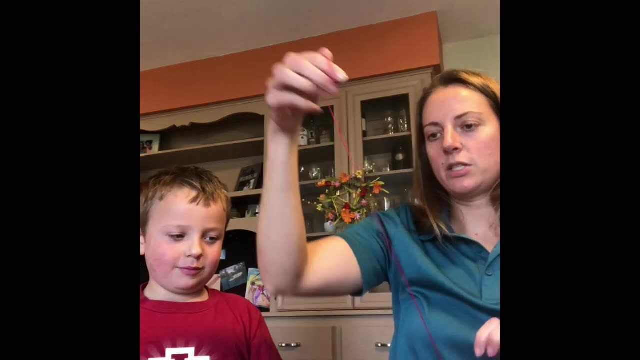 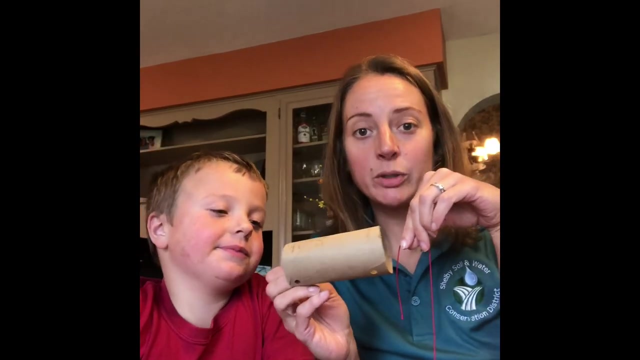 to hold this out. Jacob, Do you want to cut it About right here? Okay, I'm going to need two of them because I'm making one too, Yep, Okay. So if you have the toilet paper roll holder, you're going. 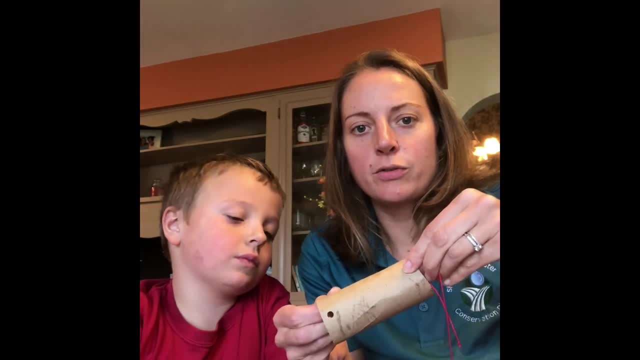 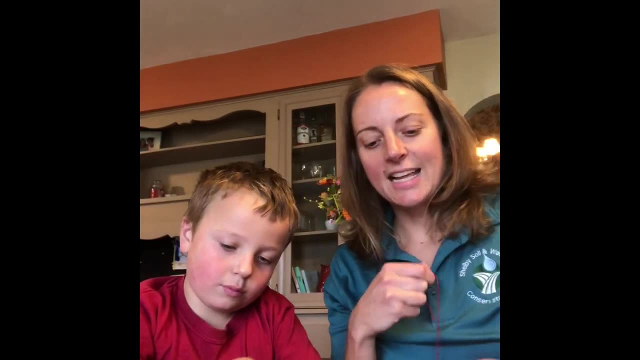 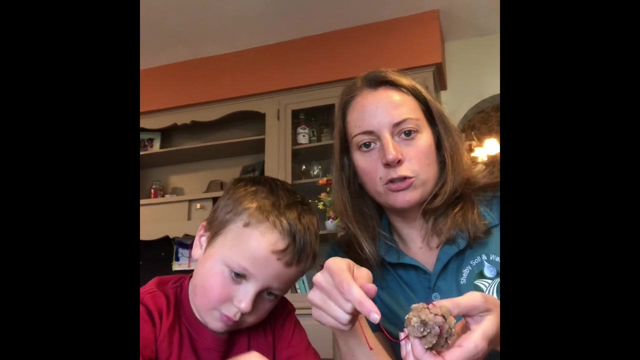 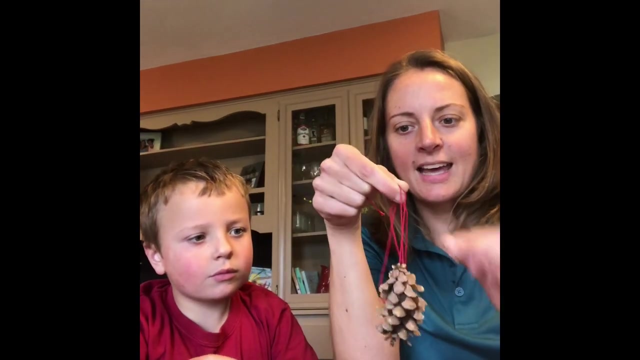 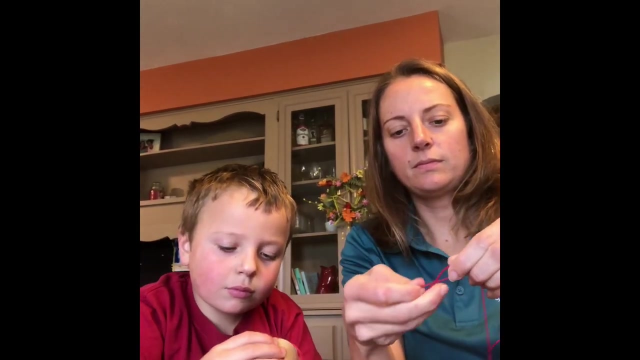 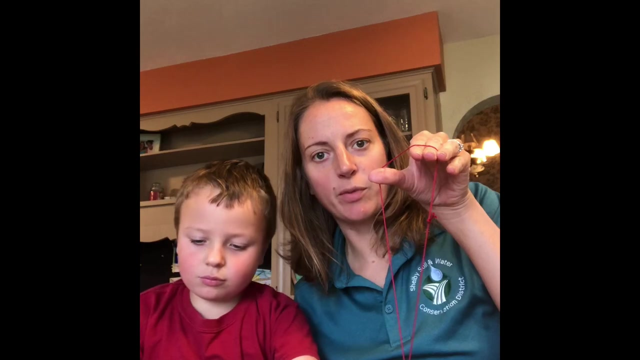 to put the yarn, punch two holes in it and put the yarn through it and tie it up. Do you want to do that? No, Take your mirror and we're going to make a. So here's the pine cone one. It's going to hang like this from a tree or a hook. 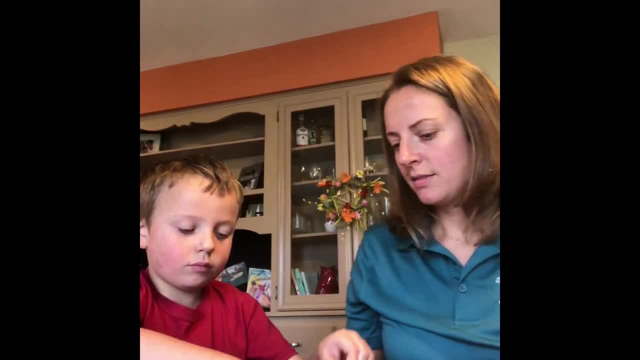 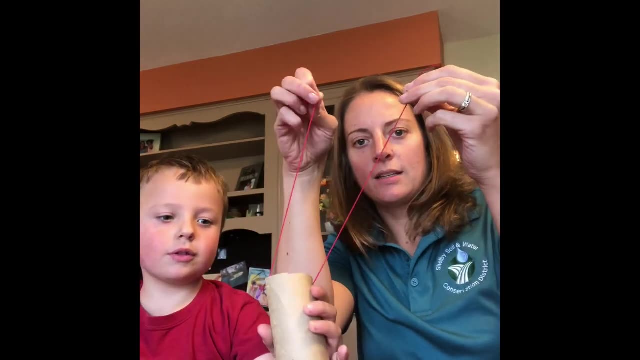 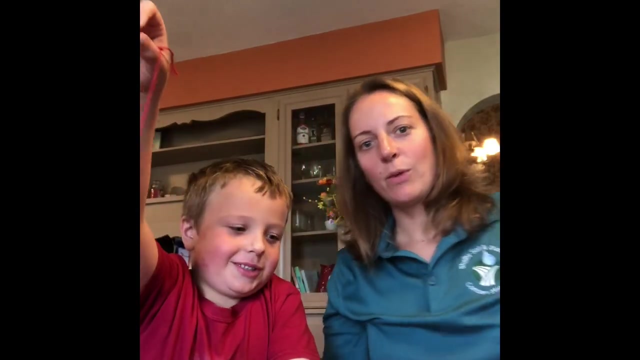 or a hook, whatever you can find. How's it coming? You got it. We just go through those two, So he would he put his this way and then we tie the top in a knot and it'll hang like that. What's the next step? Do you remember? 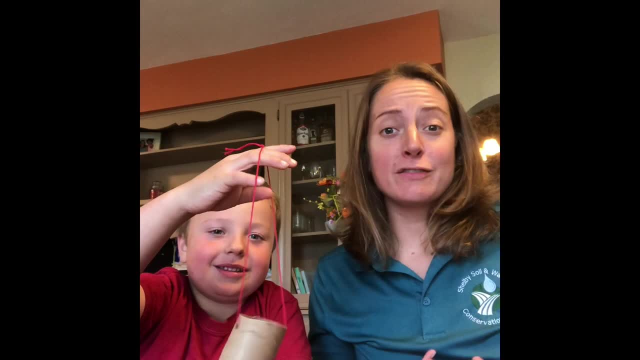 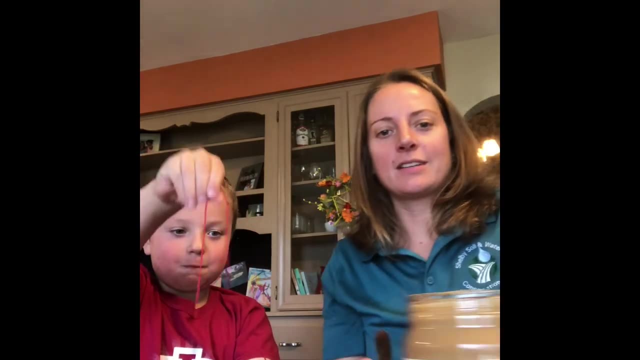 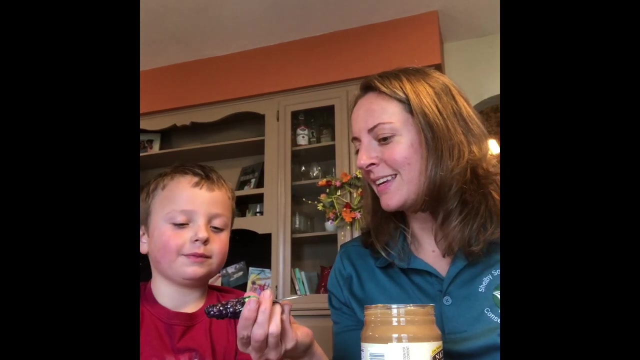 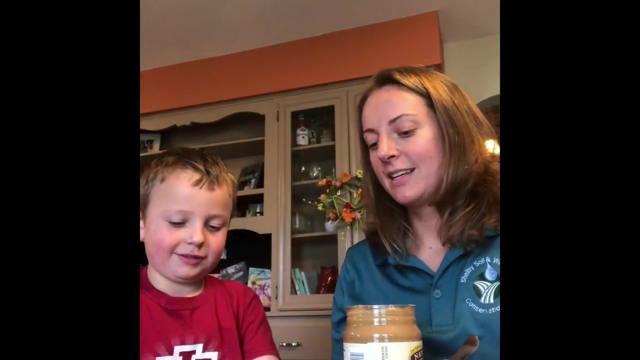 Peanut, put peanut butter on it. Peanut butter or any kind of nut butter, or, if you're allergic to nuts, maybe like hummus, something that's really sticky. So find a jar of peanut butter or whatever you're using, take a small knife and spread it around your item. Now, this is the messy part, because you don't want to put 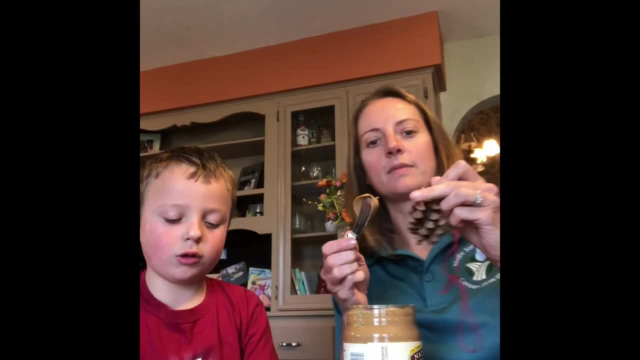 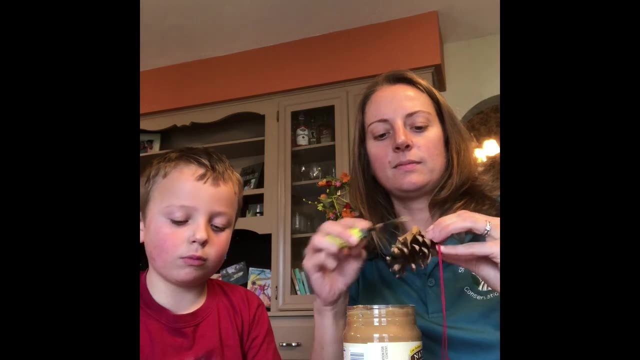 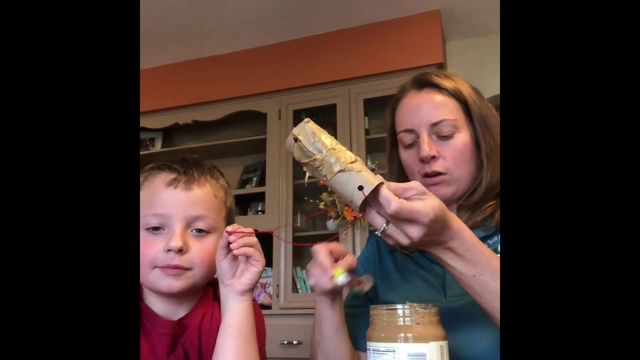 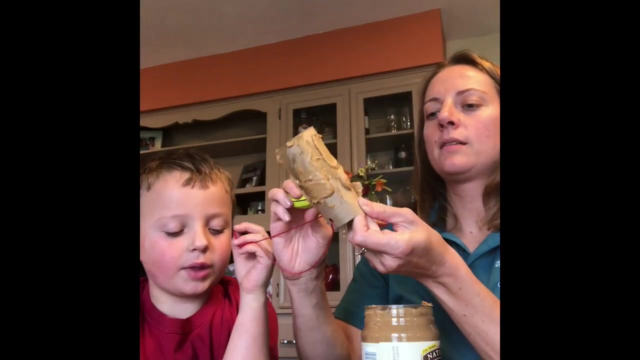 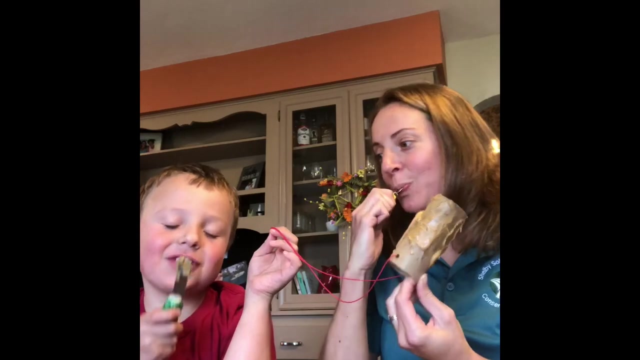 the peanut butter on the table, right? Yeah, I'm going to spread it around here on the pine cone. So once you have your peanut butter spread all around the toilet paper roll or the pine cone, then you're gonna have to eat the peanut butter. Just kidding, you totally are. Lick your knife off.